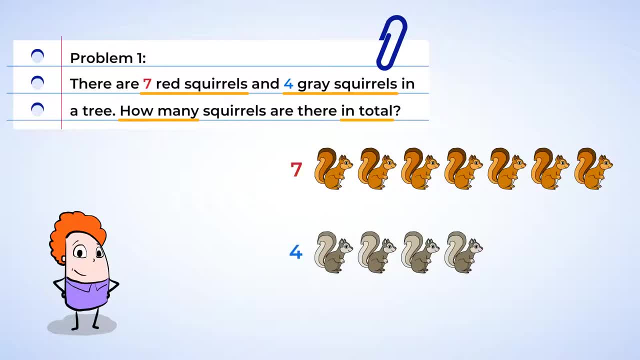 We know two of the numbers already- seven and four- And because we want to know how many there are in total, we need a plus sign to show we're adding them together: Seven plus four. Now we need an equal sign and one more number to complete the addition sentence. 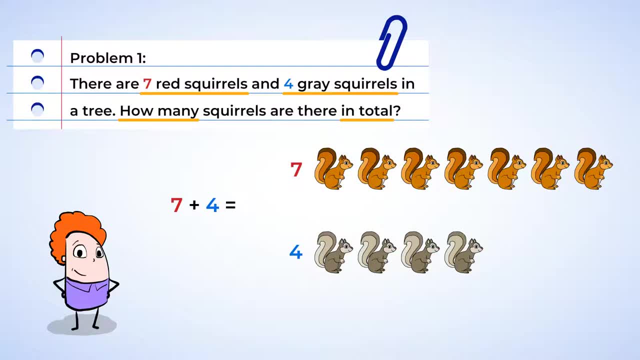 Seven plus four equals. If we don't know what the third number is yet, we can write a question mark in its place. Now our addition sentence looks like this: Seven plus four equals, And we can use the picture of the squirrels to help us. 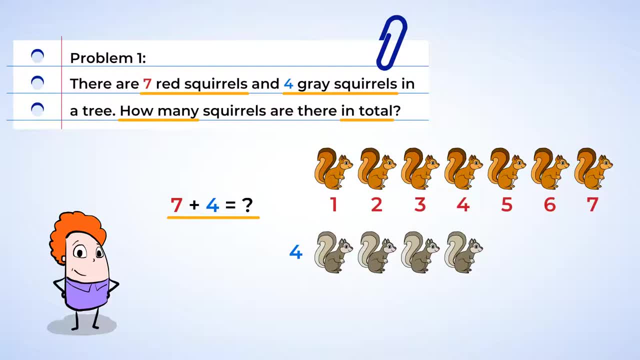 We already know there are seven red squirrels, so we don't have to count them again. We're going to start at the number seven and count up from there to add four more gray squirrels, Eight, nine, ten, eleven. Now we know that there are eleven squirrels in total. 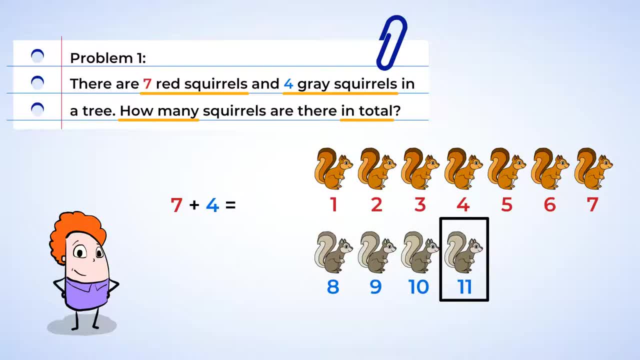 And we can replace the question mark from our addition sentence with: And our final addition sentence looks like this: Seven plus four equals eleven. Now let's read it out loud together: Seven plus four equals eleven. And you just made an addition sentence in the forest. 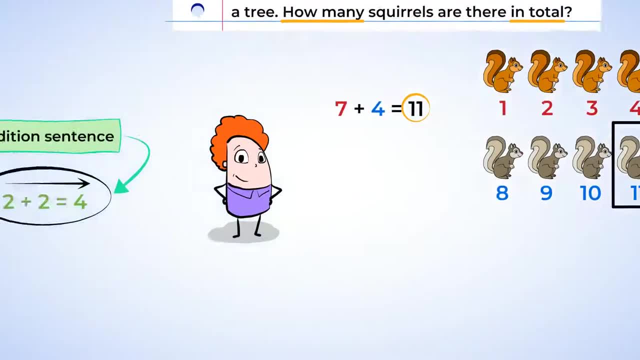 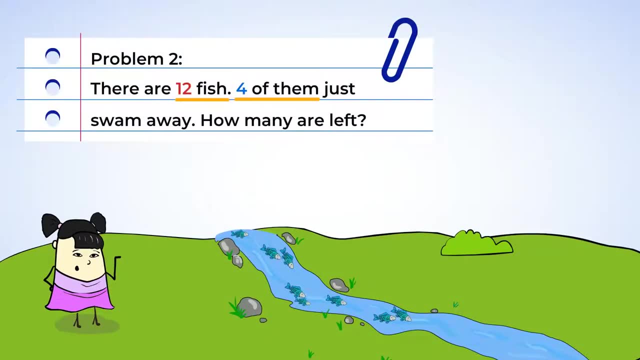 Nice job. Let's see what other animals we can find. Wow, look in the river: Twelve fish, But four of them just swam away. How many are left? Okay, so there were twelve fish when we first spotted them And now there are fewer fish because some of them swam away. 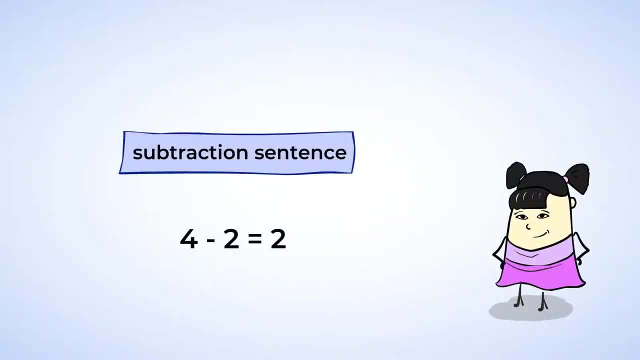 This time we'll need to make a subtraction sentence. A subtraction sentence has three or more numbers, a minus sign and an equal sign. For example, four minus two equals two is a subtraction sentence. We often use subtraction sentences to show that a number is getting smaller. 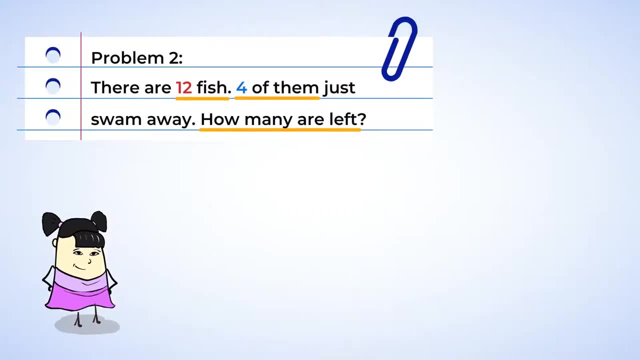 In our story we had twelve fish, but then that number got smaller. so twelve is the first number in our subtraction sentence. Of those twelve fish, four of them swam away. so we need a minus sign in the number four. Then we put the equal sign. 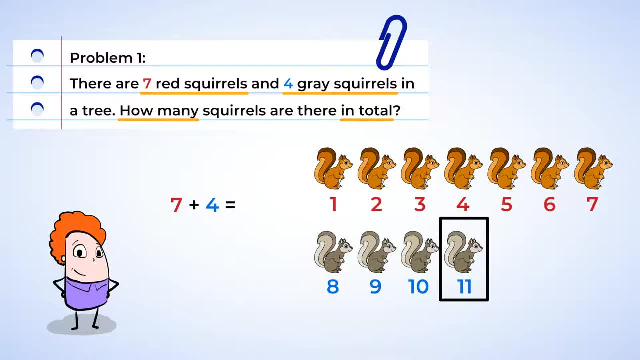 And we can replace the question mark from our addition sentence with: And our final addition sentence looks like this: Seven plus four equals eleven. Now let's read it out loud together: Seven plus four equals eleven. And you just made an addition sentence in the forest. 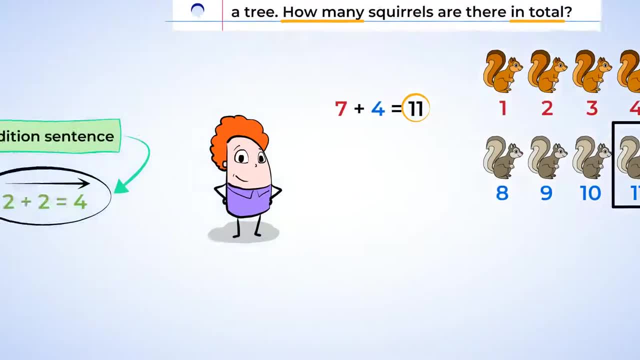 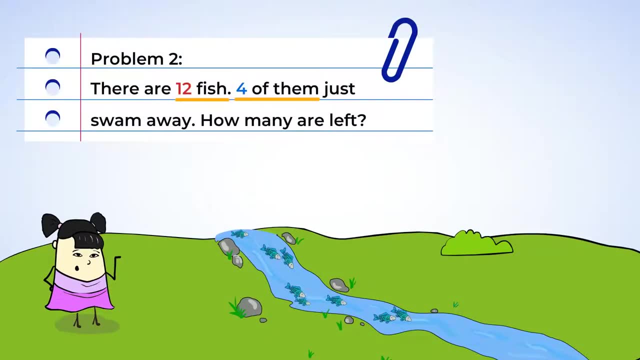 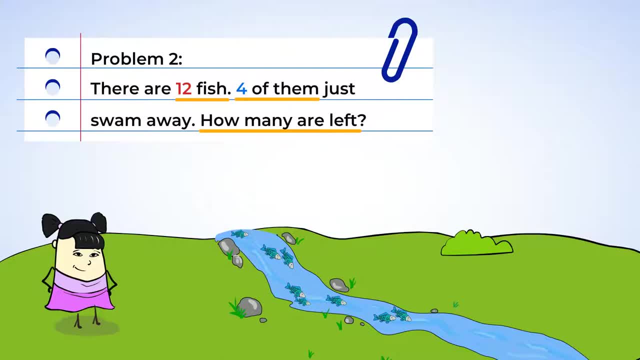 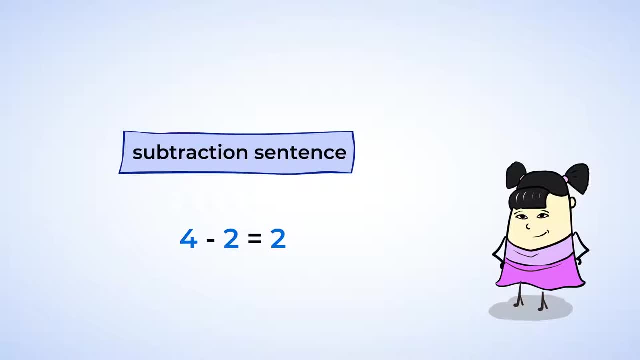 And now there are fewer fish because some of them swam away. This time we'll need to make a subtraction sentence. A subtraction sentence has three or more numbers, a minus sign and an equal sign. For example, four minus two equals two is a subtraction sentence. 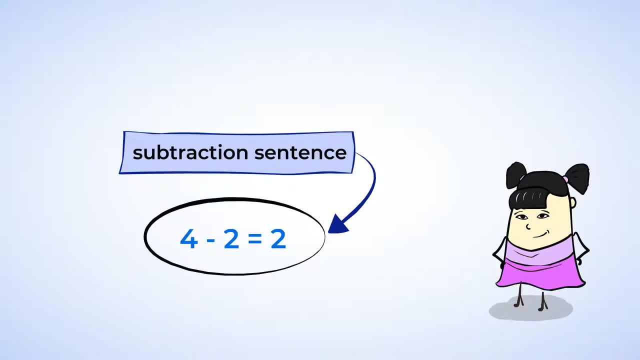 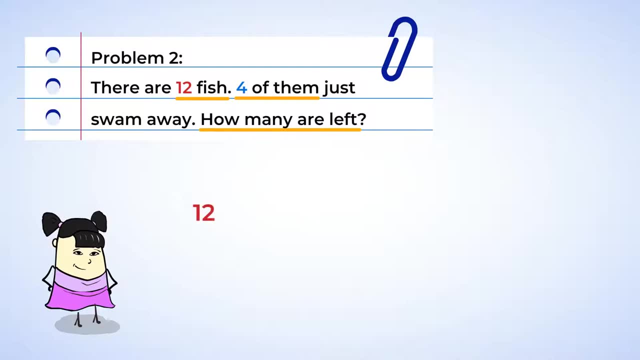 We often use subtraction sentences to show that a number is getting smaller. In our story we had twelve fish, But then that number got smaller, So twelve is the first number in our subtraction sentence. Of those twelve fish, four of them swam away. 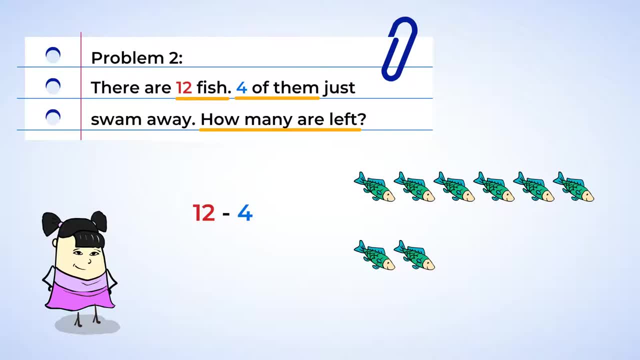 So we need a minus sign and the number four, Then we put the equal sign, But because we don't know the third number, we can put a question mark in its place, just like before. So now our subtraction sentence looks like this: 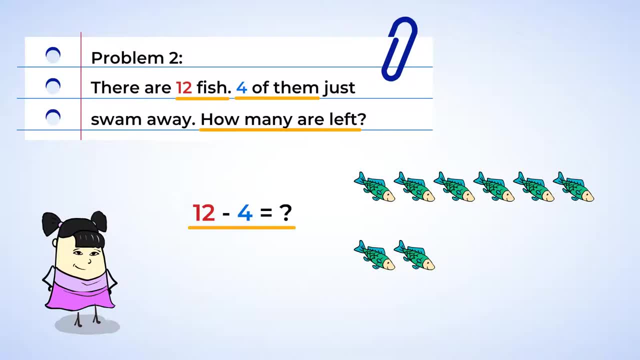 Twelve minus four equals What? We can find the answer by counting how many fish are left in the river: One, two, three, four, five, six, seven, eight. Now we can replace the question mark with the number eight. 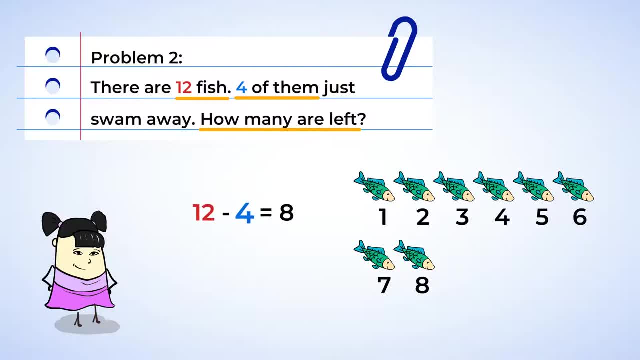 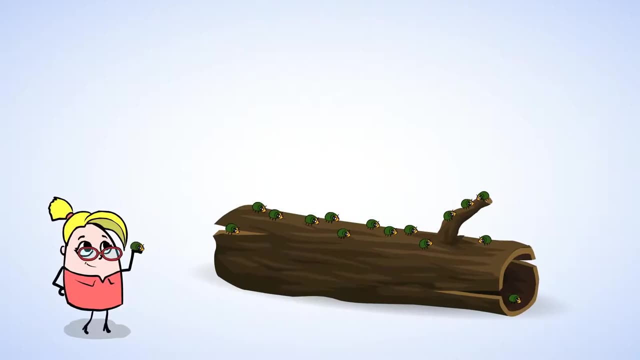 And the final subtraction sentence is: twelve minus four equals eight. Well done, We're having so much fun making math sentences in the forest, Let's try to do one more. Wow, what's that crawling over there on the log Beetles? 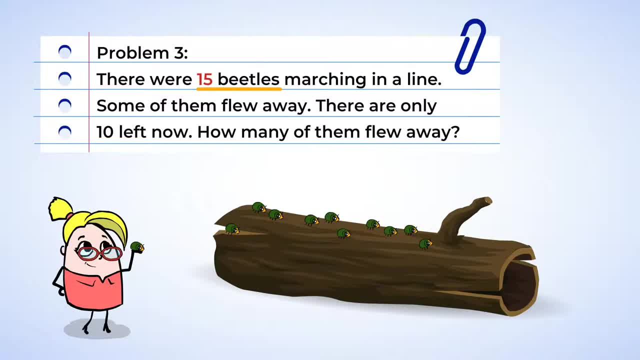 There are fifteen beetles marching in a line. Oh, some of them just flew away, And now there are only ten left. How many of them flew away Do you think we should make an addition sentence or a subtraction sentence? We can decide by asking ourselves. 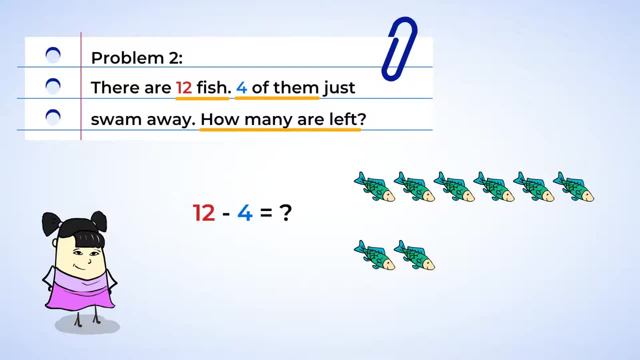 But because we don't know the third number, we can put a question mark in its place, just like before. So now our subtraction sentence looks like this: Twelve minus four equals What? We can find the answer by counting how many fish are left in the river. 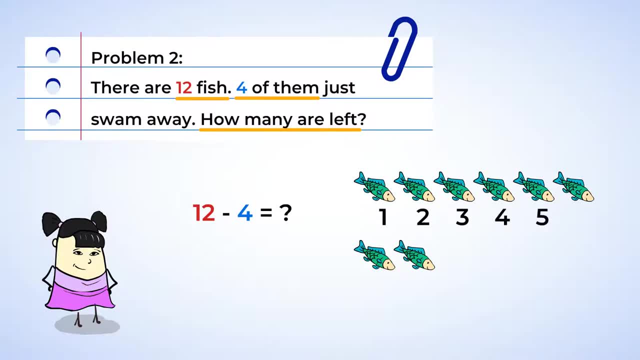 One, two, three, four, five, six, seven, eight. Now we can replace the question mark with the number eight, and the final subtraction sentence is: twelve minus four equals eight. Well done, We're having so much fun making math sentences in the forest. 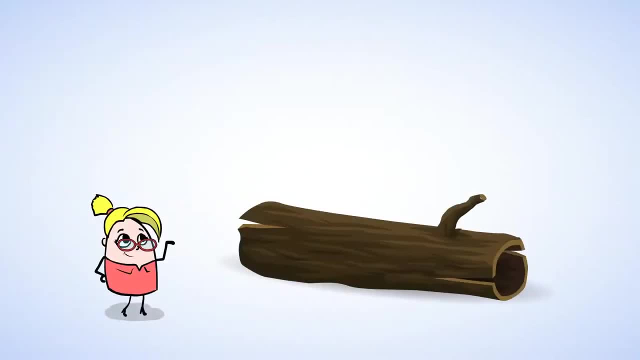 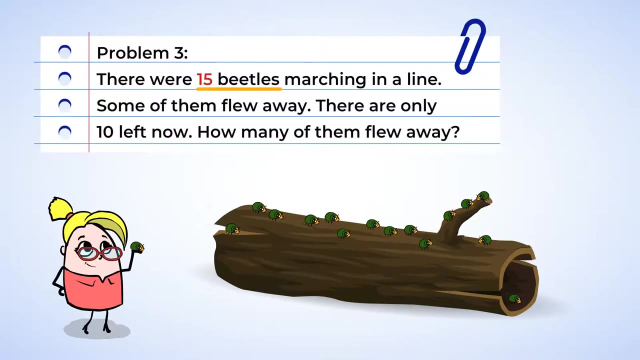 Let's try to do one more. Wow, what's that crawling over there on the log Beetles? There are fifteen beetles marching in a line. Oh, some of them just flew away and now there are only ten left. How many of them flew away? 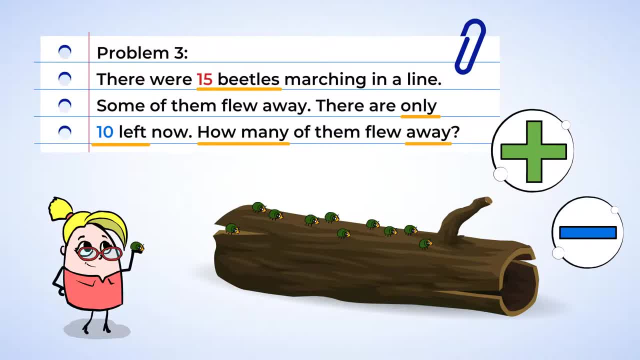 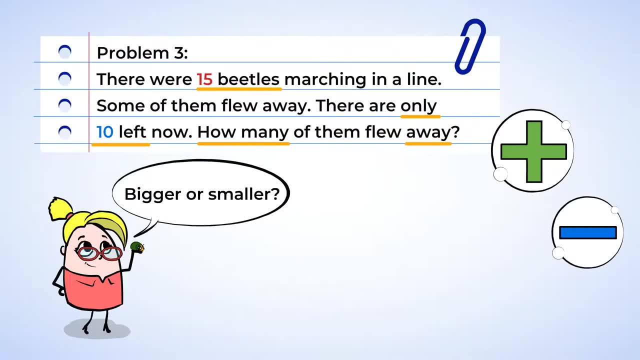 Do you think we should make an addition sentence or a subtraction sentence? Well, we can decide by asking ourselves: did the number of beetles get bigger or smaller? We can see it got smaller, and so that means we need to make a subtraction sentence. 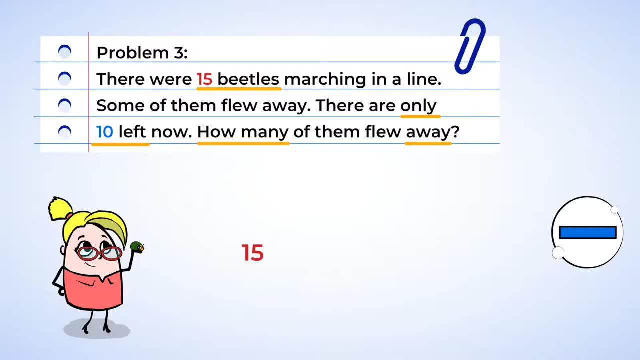 The number of beetles was fifteen, but then it got smaller, So the first number should be fifteen, followed by the minus sign. However, we don't know the next number. We have the number ten, but that's just how many beetles are still here. 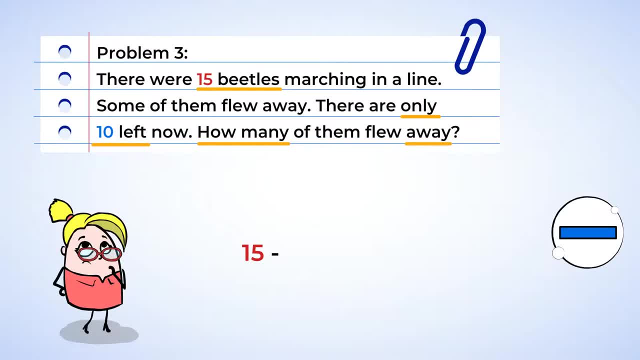 That's the answer. So what can we do? Just like before, we can use a question mark in its place. Next, we write the equals, The equals sign and the number of beetles that are left: Ten. So let's read our subtraction sentence. 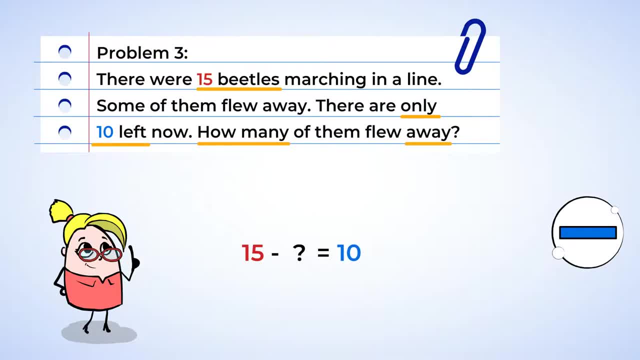 Fifteen minus what number equals ten. Let's think back to when there were fifteen beetles and let's take them away one by one. until there are only ten left To show that we're taking away, we can simply cross out a beetle. 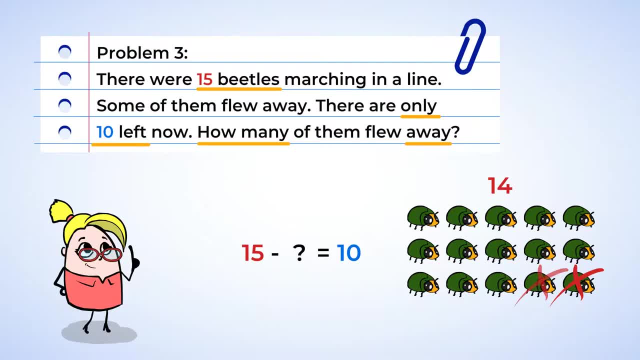 Now let's count backwards until you get to ten, Fourteen, Thirteen, Twelve, Eleven, Ten, And there are ten left. And how many were taken away? Five. Now we know that the missing number in our subtraction sentence is five. 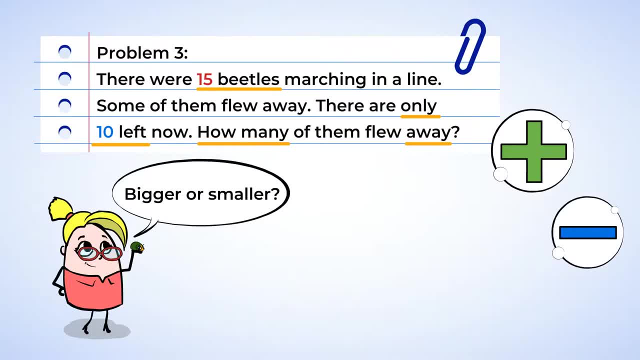 did the number of beetles get bigger or smaller? We can see it got smaller, And so that means we need to make a subtraction sentence. The number of beetles was fifteen, but then it got smaller, So the first number should be fifteen, followed by the minus sign. 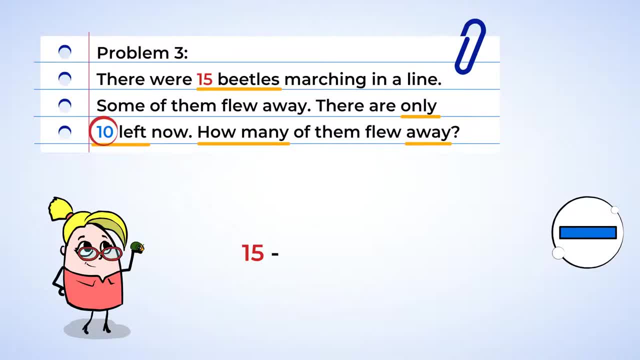 However, we don't know the next number. We have the number ten, but that's just how many beetles are still here. That's the answer. So what can we do? Just like before, we can use a question mark in its place. 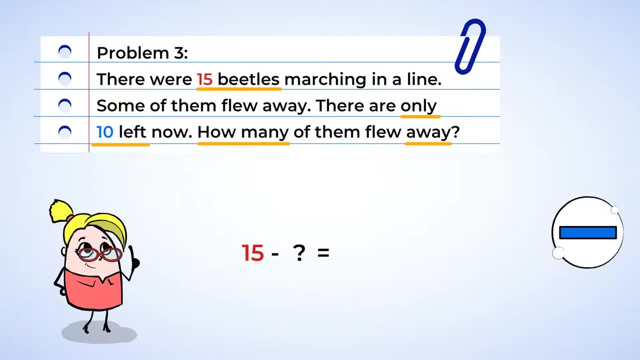 Next we write the equal sign And the number of beetles that are left: ten. So let's read our subtraction sentence: Fifteen minus what number equals ten. Let's think back to when there were fifteen beetles And let's take them away one by one until there are only ten left. 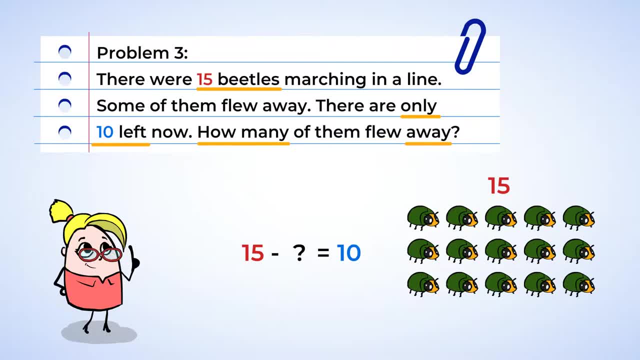 To show that we're taking away. we can simply cross out a beetle. Now let's count backwards until you get to ten, Fourteen, thirteen, twelve, eleven, ten, And there are ten left. And how many were taken away? 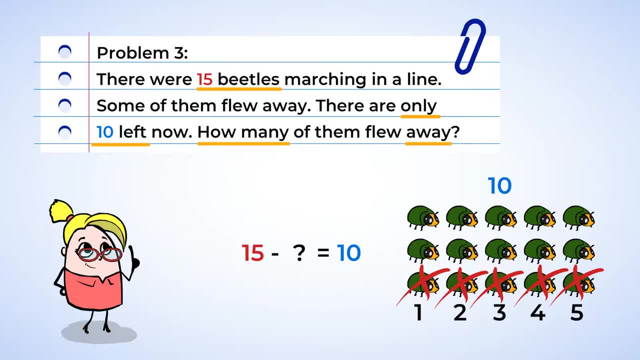 Five. Now we know that the missing number in our subtraction sentence is five. Fifteen minus five equals ten. We did it. We made another subtraction sentence. Let's review what we learned today on our math field trip in the forest. When putting two numbers together, like the seven red squirrels and the four gray squirrels, 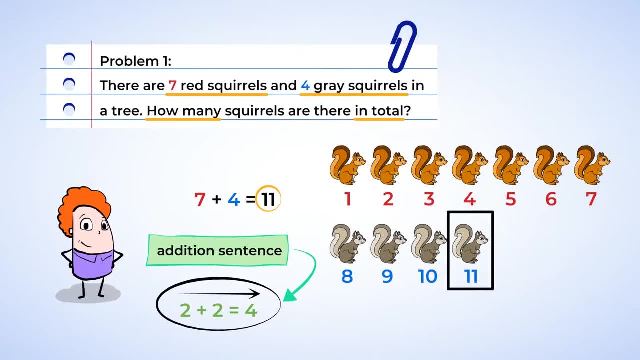 we can represent this with an addition sentence. We write the number of the first group- a plus sign, the number of the second group, an equal sign, and the number of both groups together. And when a number gets smaller, like the fish in the river, 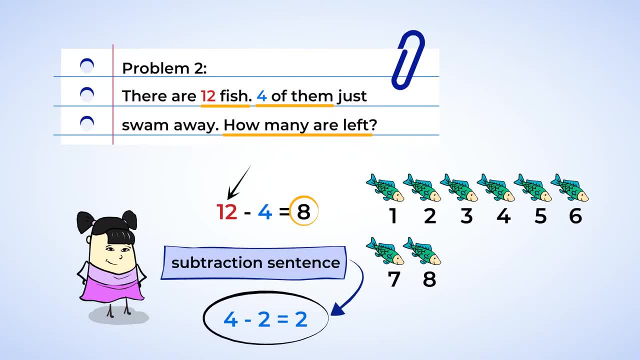 we can show this with a subtraction sentence. First we write the total number, a minus sign, how many were taken away, an equal sign, and then how many were left. If you don't know a number, you can just write a question mark in its place. 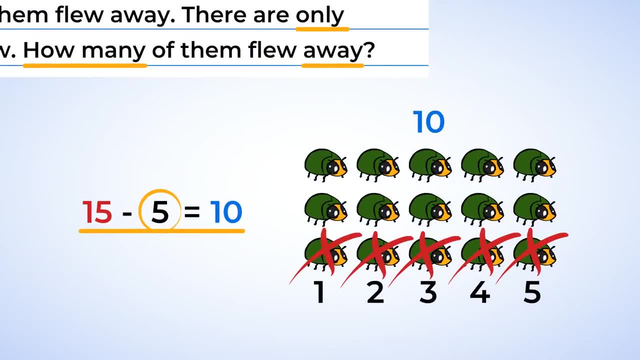 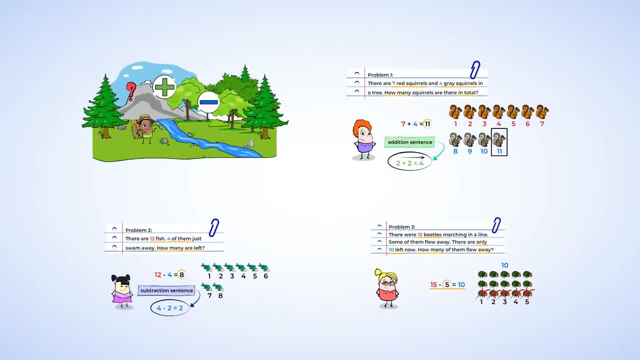 And when you're ready to find out what the missing number is, you can use pictures to help you Count up when adding or cross out when subtracting. Great work today. I can't wait to go on more mighty field trips with you.